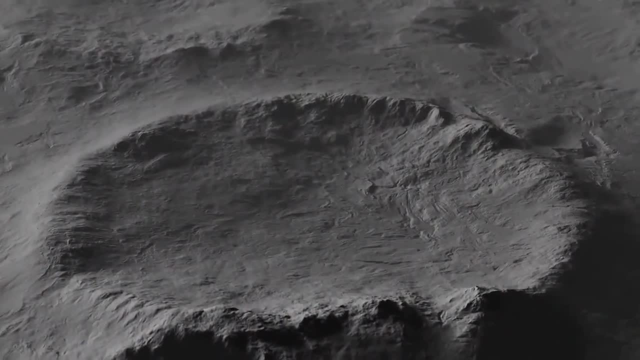 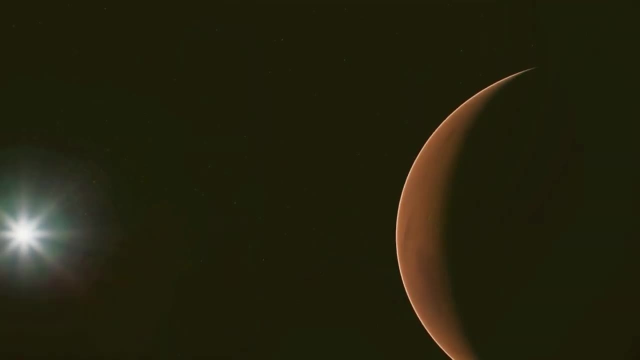 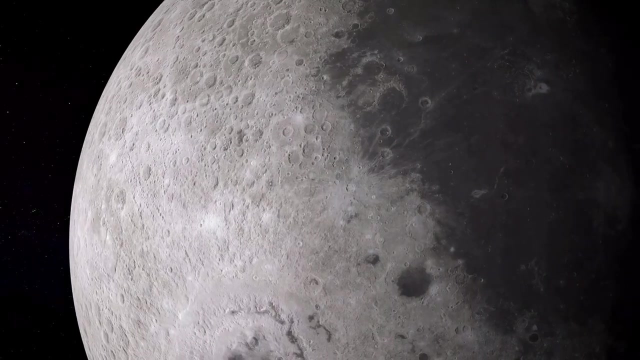 These moons were discovered in the late 19th century, when the planet was first discovered. The names Phobos and Deimos come from Greek mythology, representing fear and dread, fitting companions for Mars, the god of war. Fascinatingly, it is believed that these 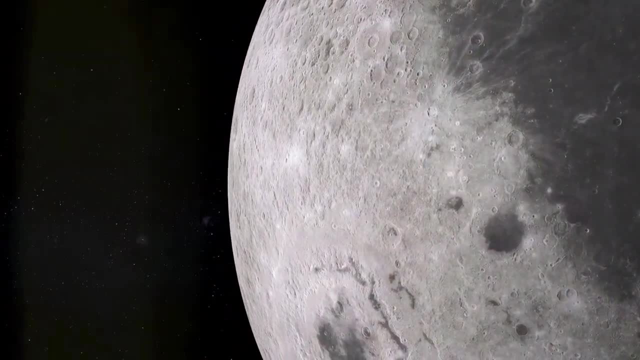 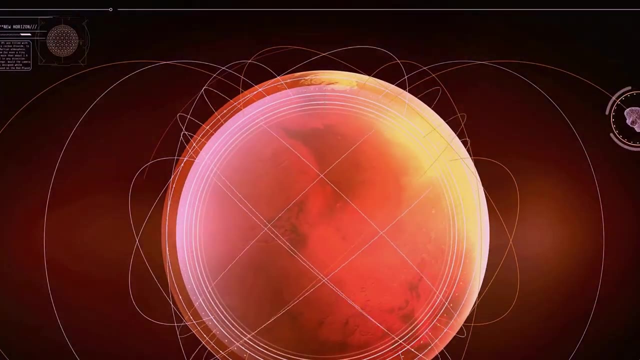 moons are not native to Mars, but rather they are captured asteroids. This theory is supported by their composition, similar to that of asteroids found in the asteroid belt, but not as a whole. The names. Phobos and Deimos are not native to Mars, but rather they are. 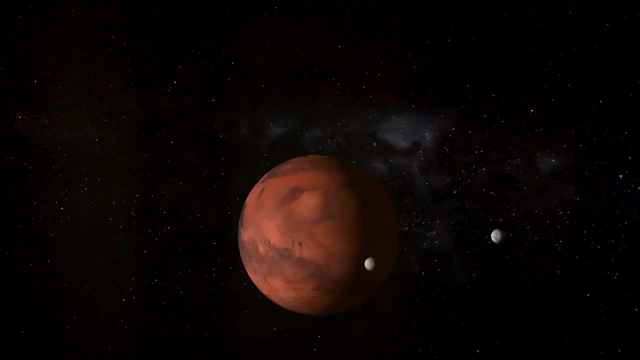 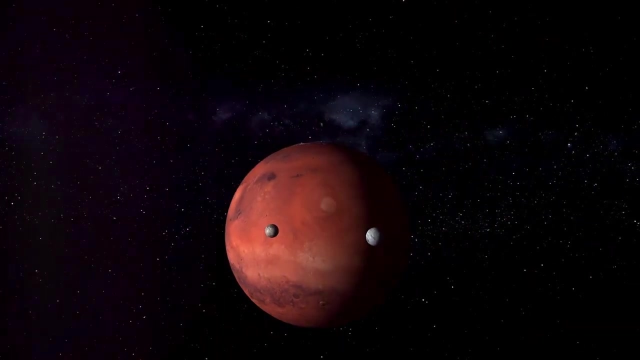 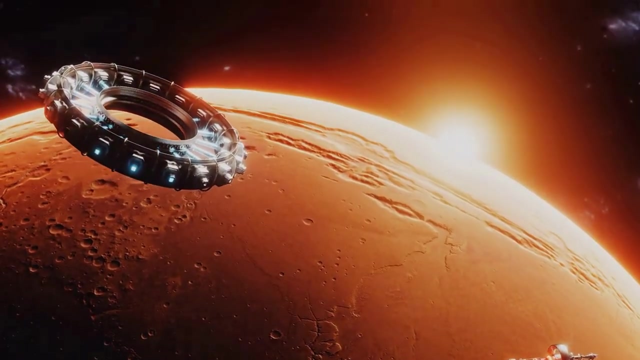 between Mars and Jupiter. Their small size and irregular shape, coupled with their close proximity to Mars, make them intriguing subjects of study to understand the early solar system. NASA even has plans to send missions to these moons in the near future, While Mars may not. 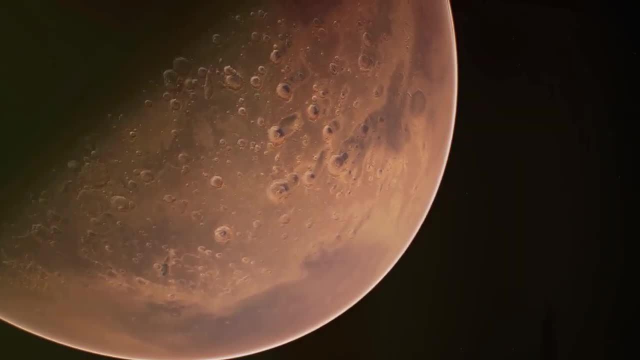 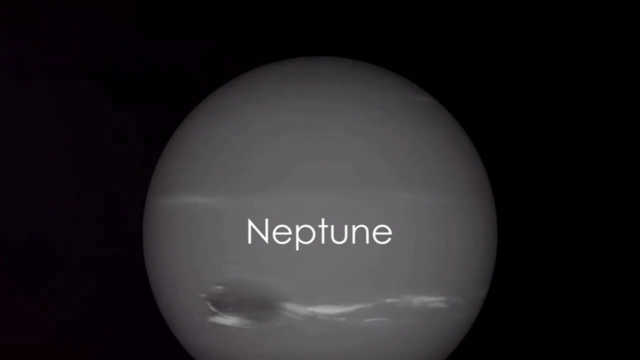 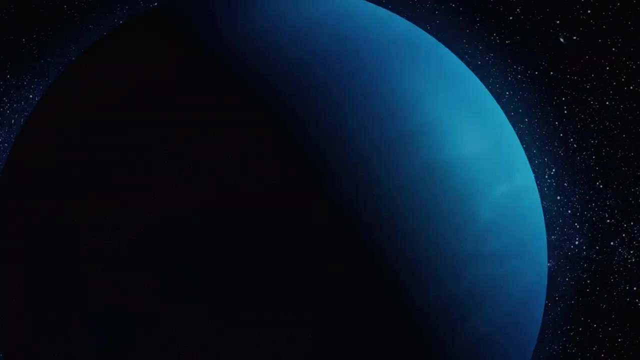 boast a high number of moons. its two satellites are fascinating in their own right. Moving on, we find Neptune, claiming the fourth star. This gas giant crowned with a striking blue hue is home to 14 moons. Each one of these celestial bodies has a story to tell, a secret to reveal about the farthest planet from the Sun. 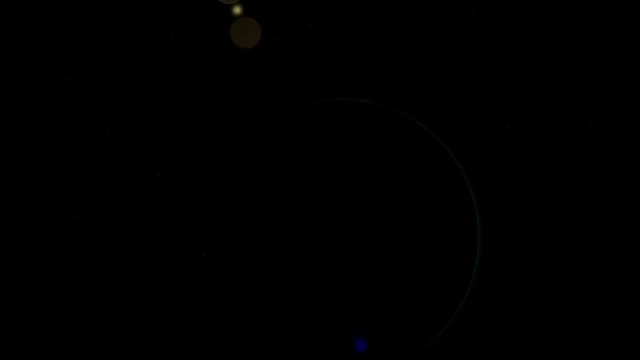 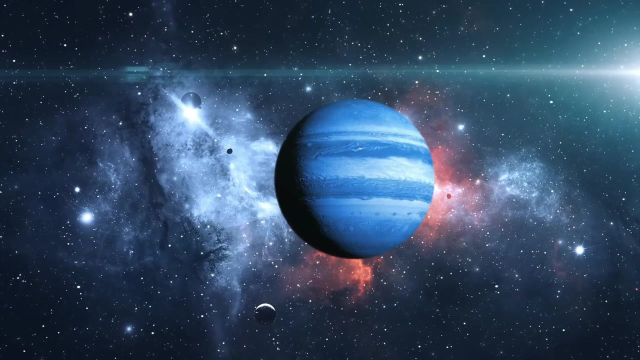 in our solar system. The largest of Neptune's moons, Triton, is a sight to behold. Named after the Greek sea god, Triton is not only the biggest, but also the most intriguing. It's a moon that marches to the beat of its own drum, and it's the largest moon in the world. It's the largest moon. 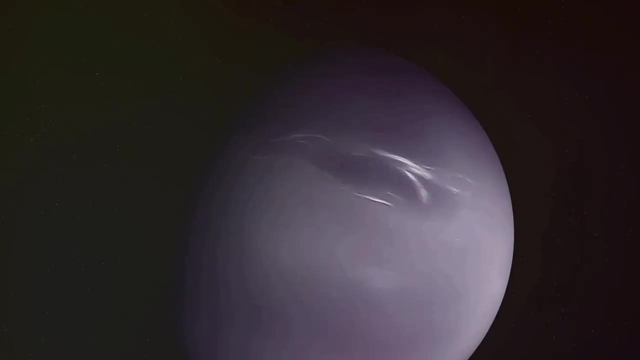 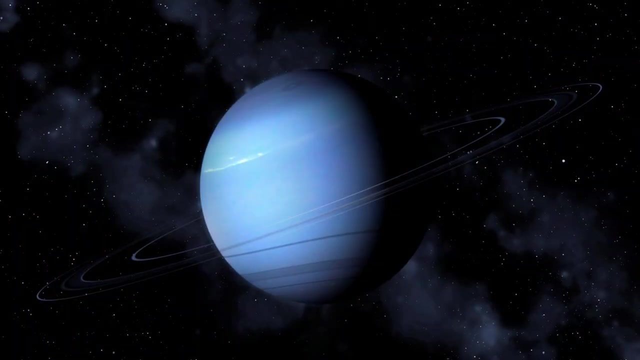 in the world and it's the largest moon in the world. It's the largest moon in the world, Some quite literally. You see, Triton follows a retrograde orbit, meaning it moves in the opposite direction to Neptune's rotation. In the cosmic ballet of the universe, Triton is a. rebellious dancer, defying the norm and adding a dash of mystery to Neptune's celestial family. But Triton is not alone. Thirteen other moons orbit Neptune, each one smaller than the last, From Nereid, the third largest, with its highly eccentric orbit, to tiny Nereid, the innermost moon. Neptune's moons are as diverse. 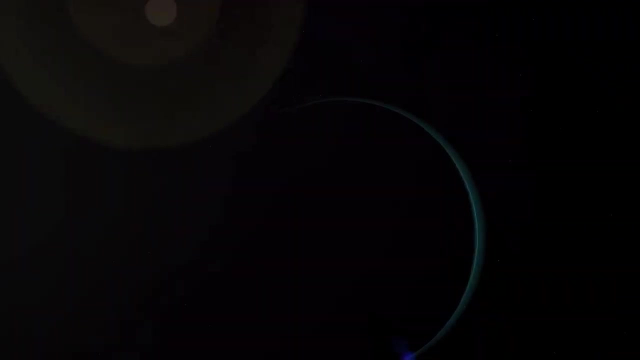 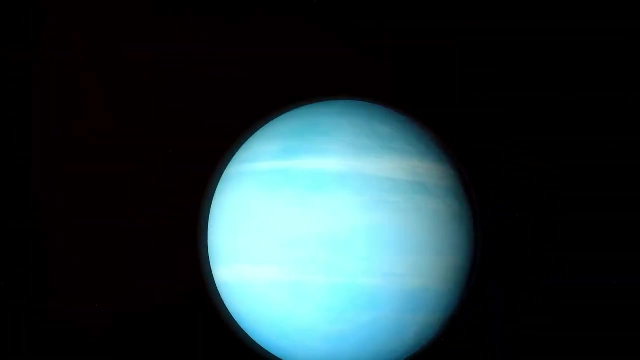 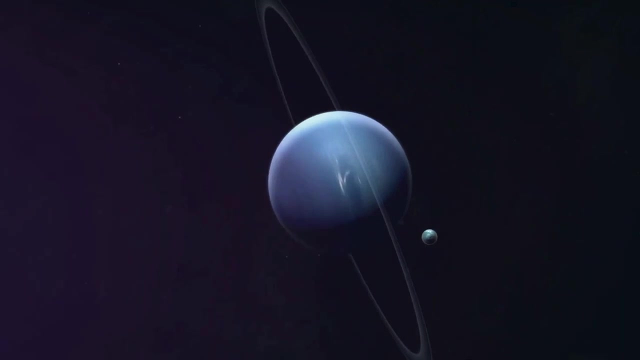 as they are numerous. These moons, far from being mere satellites, offer tantalizing clues about Neptune, its history and its place in our solar system. They serve as reminders that even at the edge of our solar system there are wonders waiting to be discovered, secrets waiting to be revealed. 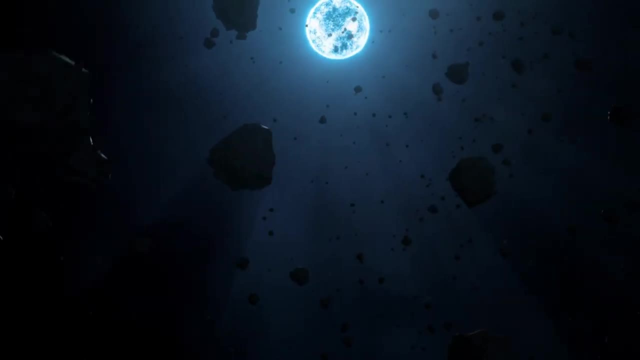 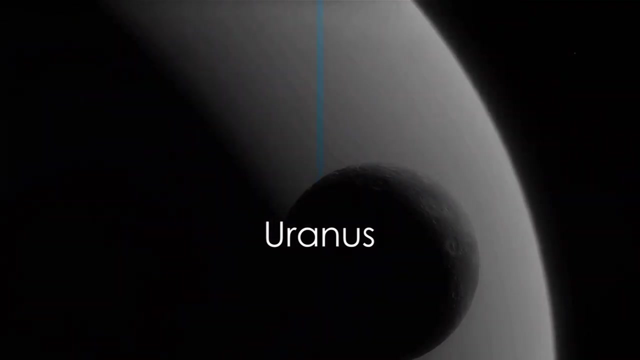 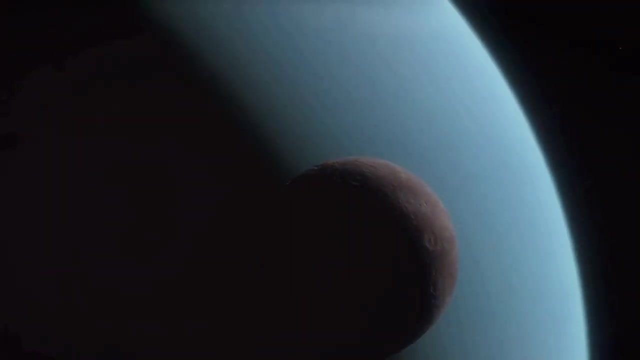 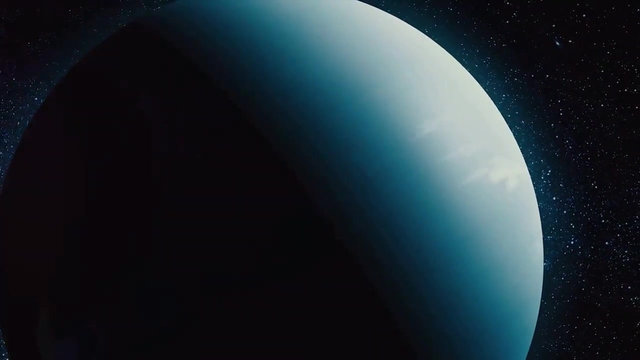 Despite its distance from the Sun, Neptune's moons make for some intriguing study. Next up, at the third spot, we have Uranus. As we journey into the celestial realm of Uranus, the seventh planet from the Sun, we find ourselves in the company of a staggering 27 known moons, This icy giant named after the. 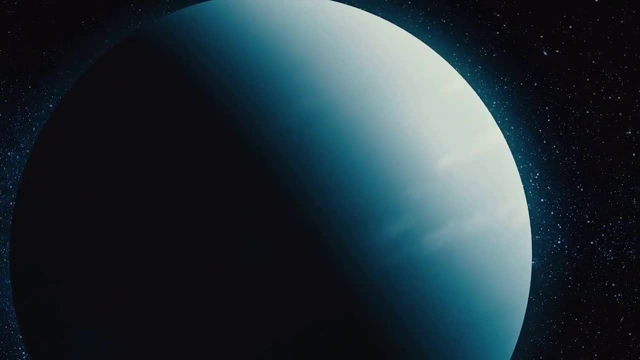 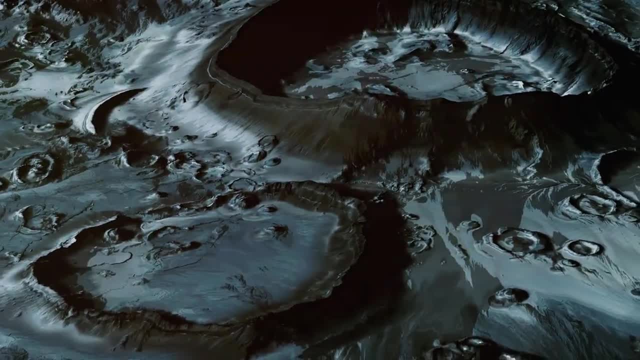 Its surface is a chaotic mix of terrains, leading some to believe it may have been shattered and reassembled. Next we have Ariel, with its system of valleys, wastes of offcerements, and and and canyons, suggesting geological activity in its past. 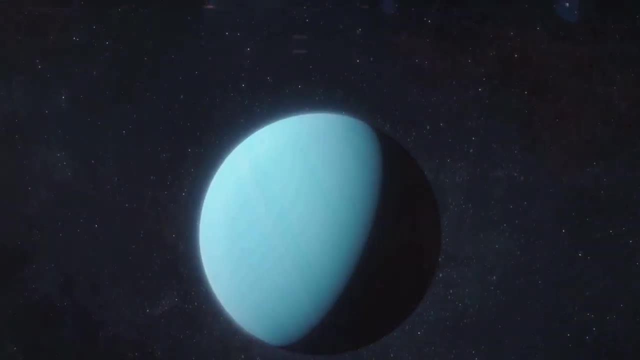 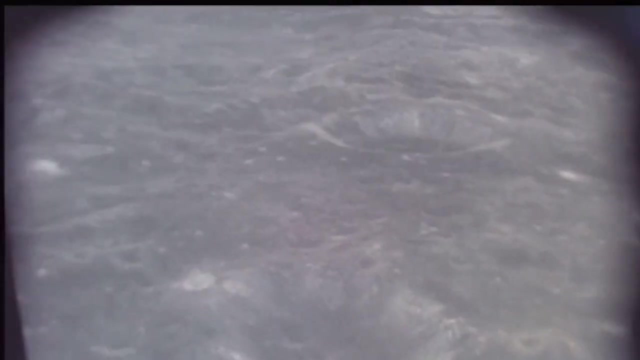 Then there's Umbriel, the darkest of the five, its surface a mystery covered in a layer of dark material. Titania, the largest moon of Uranus, boasts deep valleys and fault scarps, a testament to its tectonic past. 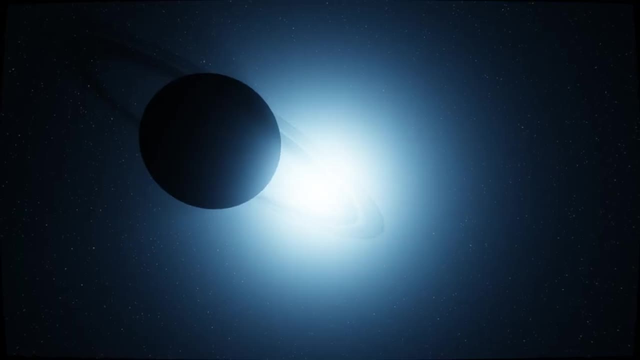 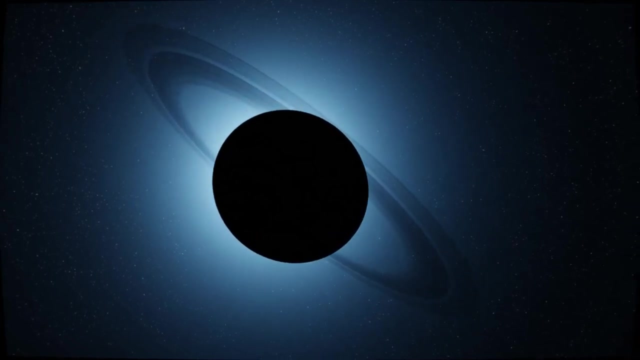 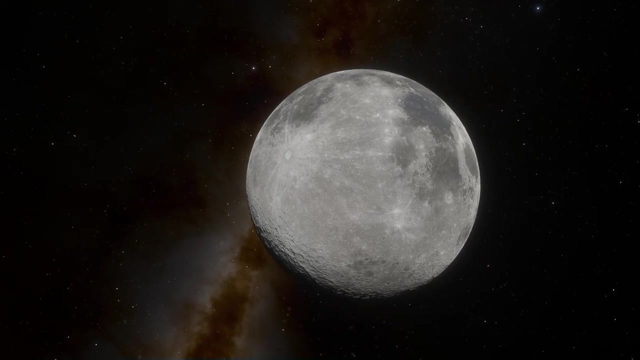 Lastly, Oberon, the outermost of the major moons, is home to an old, heavily cratered surface indicating a long history of cosmic impacts. These moons, with their unique features, offer a glimpse into the diverse processes that shape the celestial bodies within our solar system. 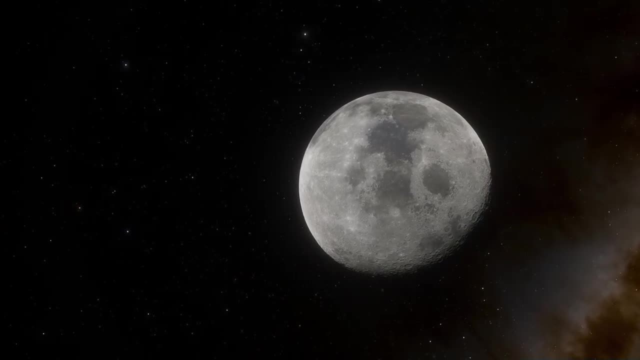 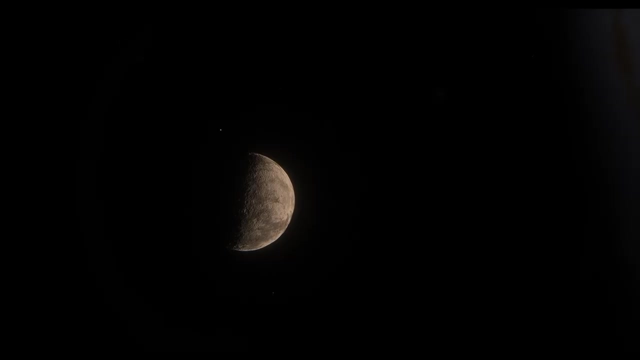 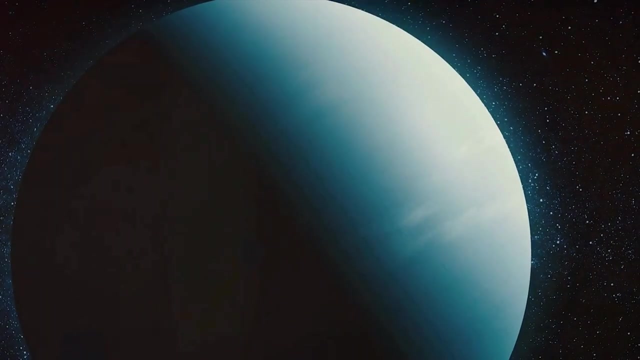 Their presence around Uranus hints at the intriguing complexities of planetary science and the ongoing evolution of these distant worlds. Uranus, with its family of 27 moons, certainly adds to the diversity of our solar system. Almost at the top, in the second spot, we find Saturn. 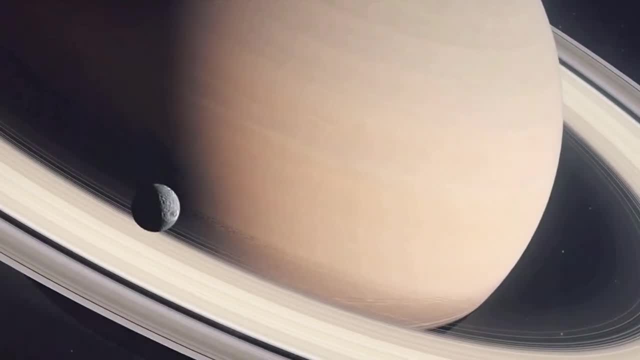 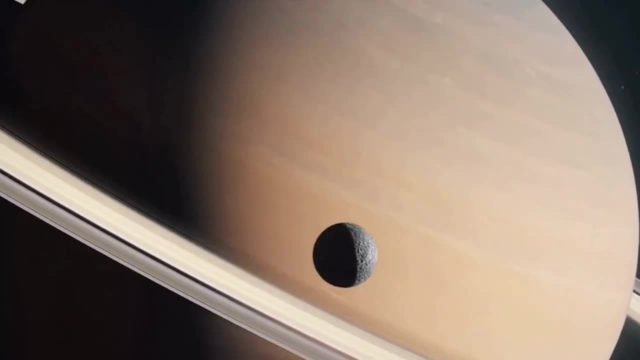 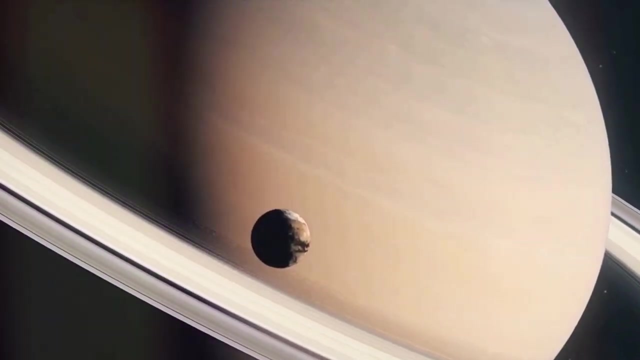 Saturn, the sixth planet from the Sun, is a celestial spectacle with a stunning collection of moons. As of today, this gas giant boasts 82 known moons, each with its own distinct characteristics and quirks. Yes, you heard it right: 82 moons. 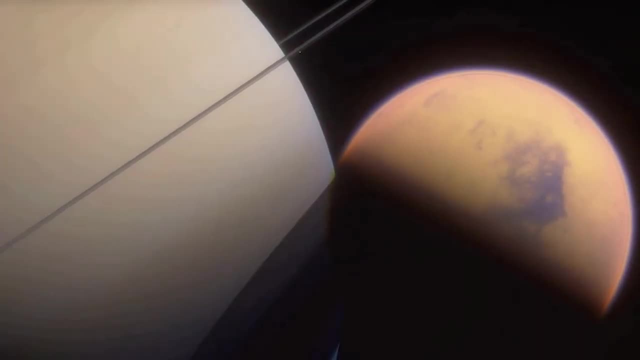 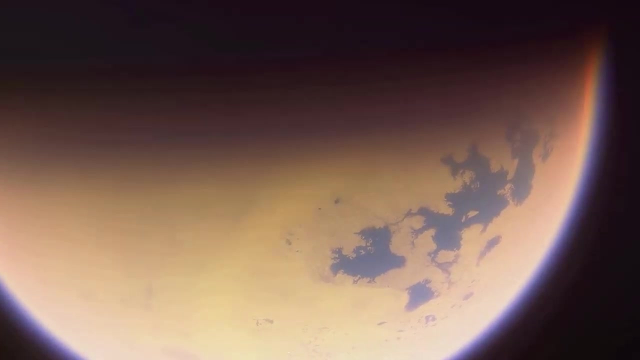 Now let's focus on the star of the show, Titan. Titan is the star of the solar system. Titan is not just any ordinary moon. It's the second-largest moon in our solar system, only slightly smaller than Jupiter's Ganymede. 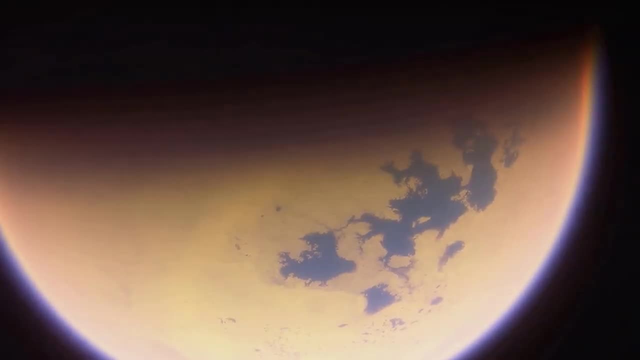 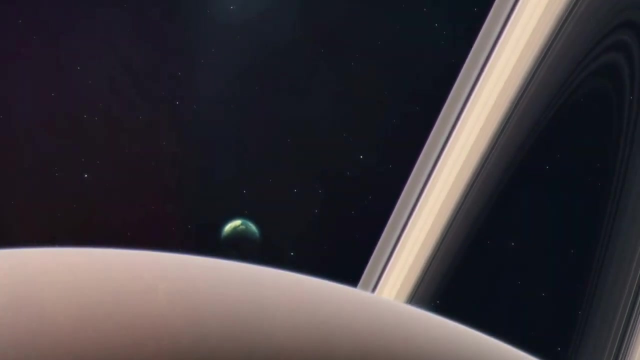 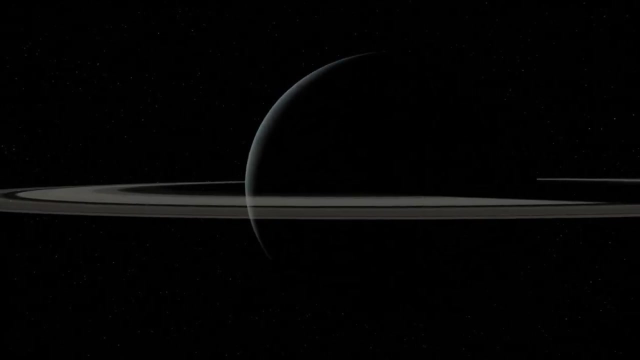 But what makes Titan truly stand out is its complex atmosphere. You see, Titan is the only moon in our solar system to have a dense atmosphere, and it's even thicker than Earth's. This atmosphere is primarily composed of nitrogen, with traces of methane and ethane. it's so. 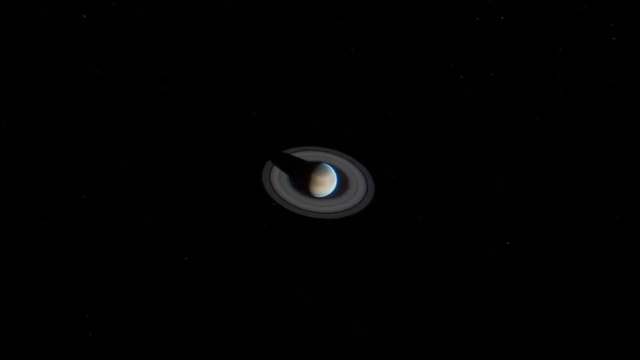 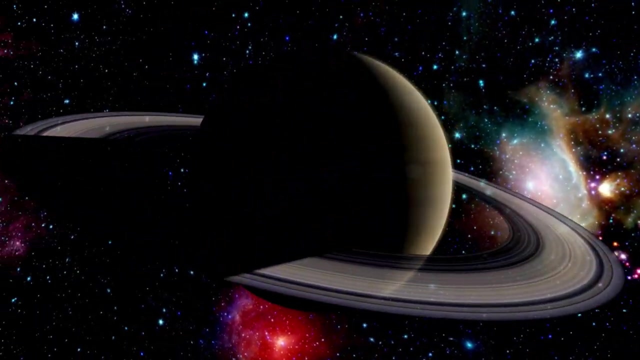 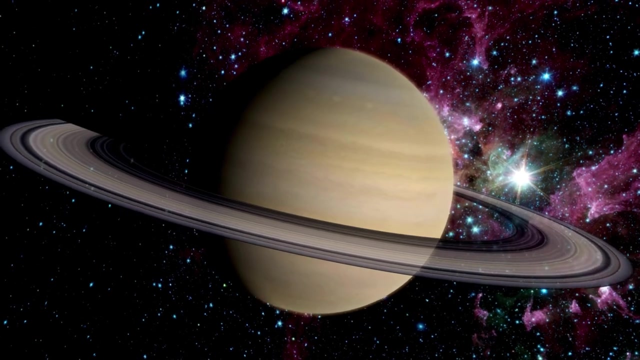 thick that it obscures our view of the moon's atmosphere. Titan's atmosphere is so complex that it even has its own weather system. It experiences seasons, just like we do on Earth, and it has clouds that rain methane and ethane. This exotic rain seeps into the ground, forming vast lakes and rivers on Titan's surface. 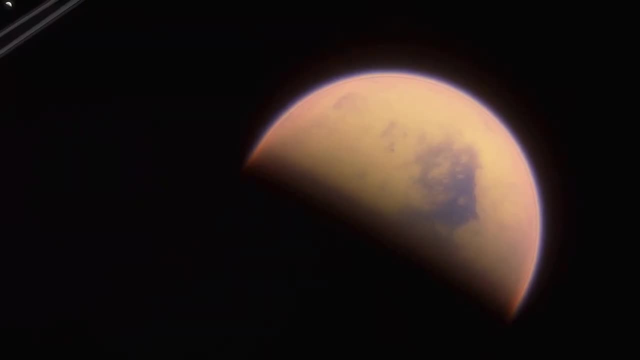 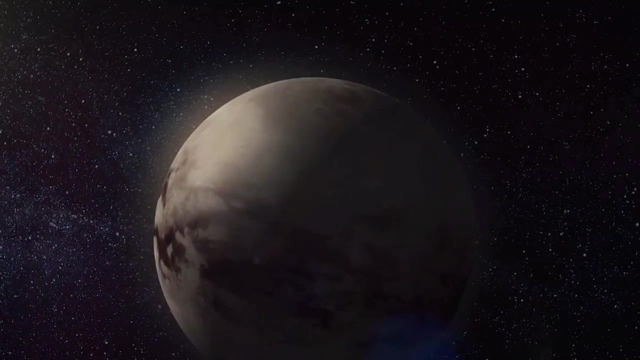 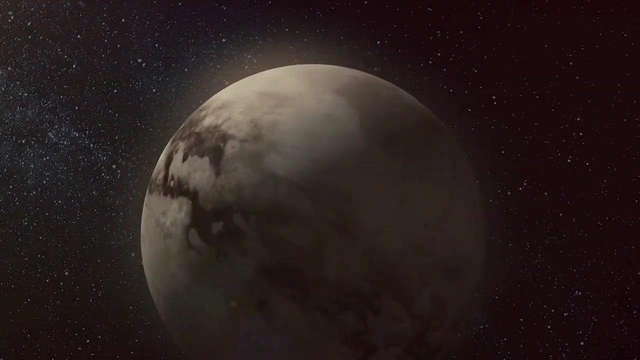 In fact, Titan is often compared to a primitive Earth, offering a glimpse into our planet's past. It's a tantalizing destination for future space exploration missions, with scientists eager to uncover its secrets. Now let's not forget the other eighty-one moons of Saturn. 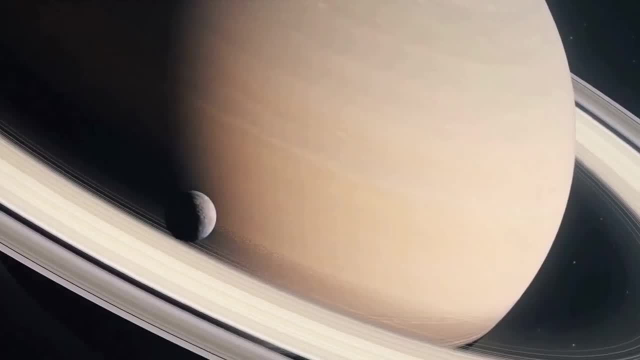 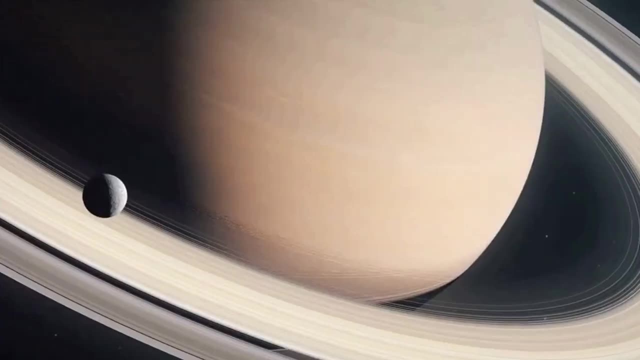 Some are tiny, just a few kilometers across, while others, like Rhea and Iapetus, are several hundred kilometers in diameter. Each one of these moons adds a unique piece to the fascinating puzzle that is Saturn. Saturn, with its dazzling rings and multitude of moons, is the only moon in our solar system. 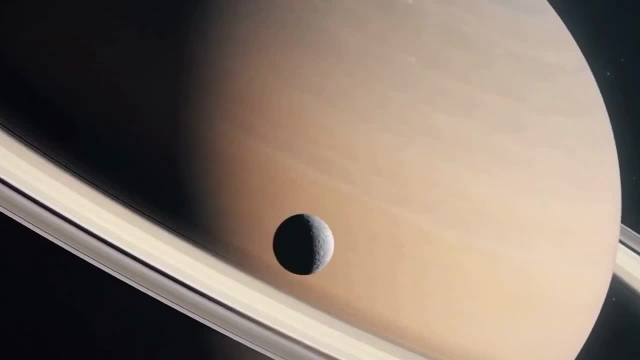 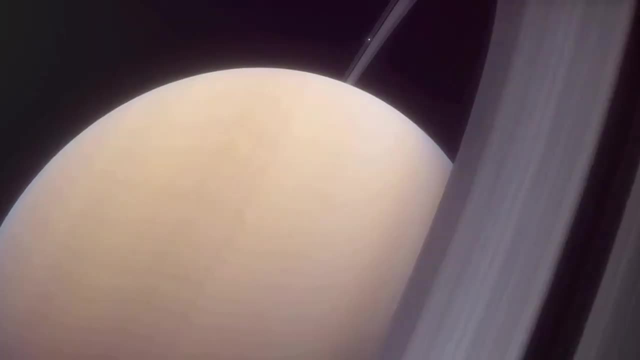 to have a vast atmosphere. A multitude of moons is truly a gem of our solar system, From its largest moon, Titan, with its complex atmosphere and weather system, to its smallest moonlets, each contributing to the planet's unique character. Saturn never ceases to amaze. 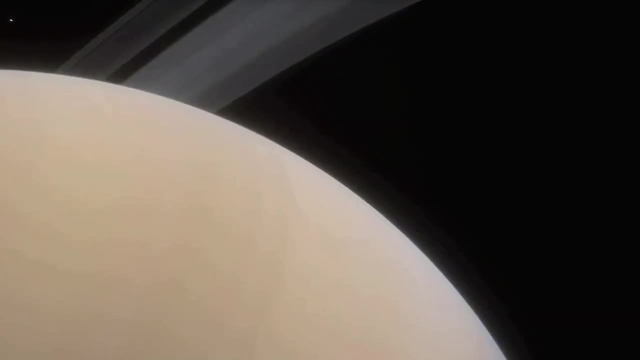 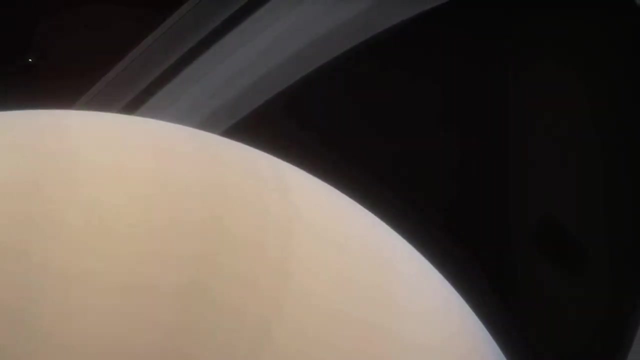 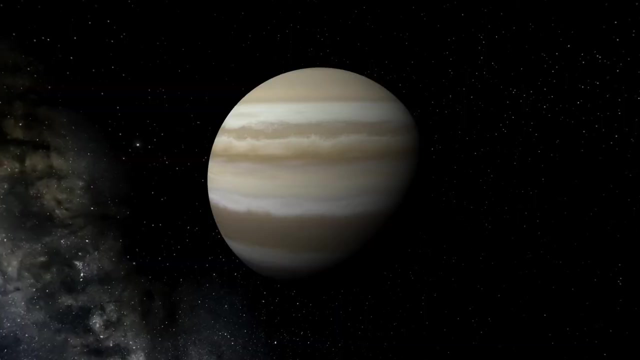 and inspire. Saturn, with its dazzling rings and multitude of moons, is truly a gem of our solar system. And now, at the top spot… We have… One of the planets, Jupiter. If you thought Saturn was impressive with its sixty-two moons, prepare to be astounded. 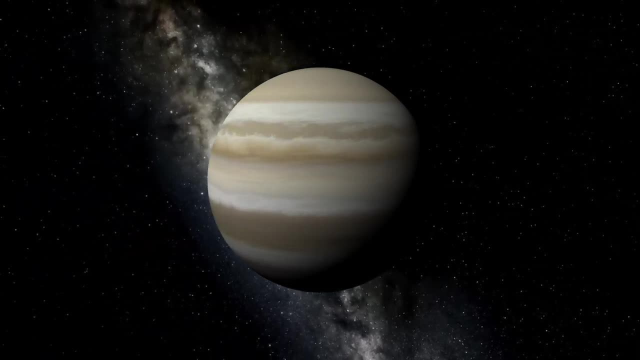 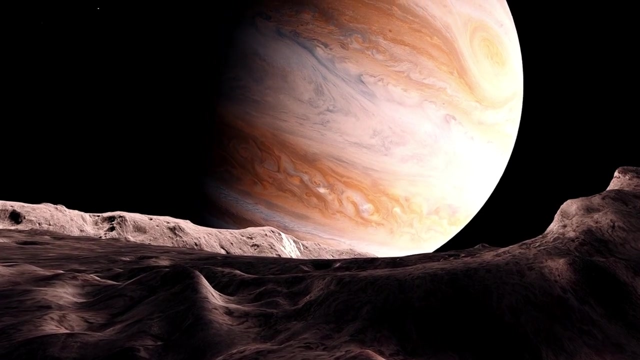 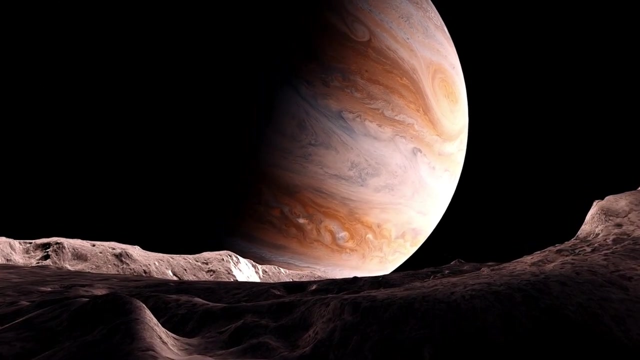 Jupiter, the largest planet in our solar system, is home to a staggering seventy-nine known moons. That's right, seventy-nine. It's a celestial royal court fit for a king. But among this multitude of satellites, four stand out, known as the Galilean moons, named 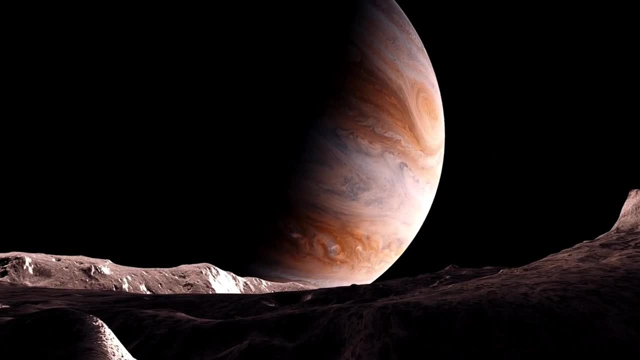 after their discoverer, Galileo Galilei. The Galilean moons are known as the Galilean moons named after their discoverer, Galileo Galilei. These are Io, Europa, Ganymede and Callisto, each with their unique characteristics and 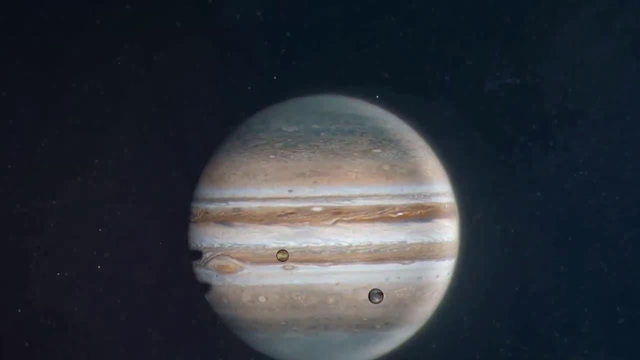 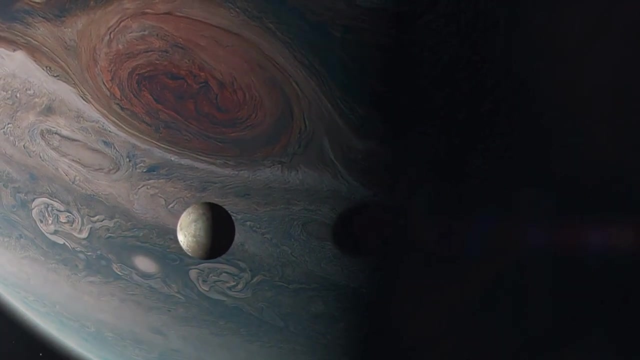 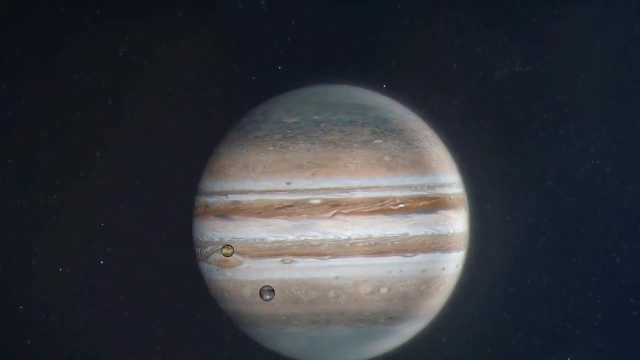 mysteries that continue to fascinate scientists and space enthusiasts alike. First up is Io, the most volcanically active body in our solar system. This moon is a fiery world of molten rock and sulfurous plumes, painting a vibrant, ever-changing landscape that's nothing short of otherworldly. 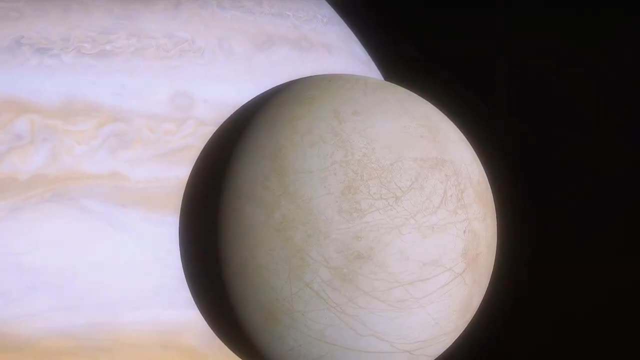 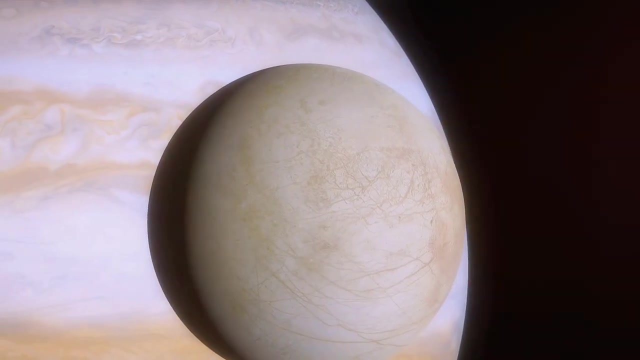 Next we have Jupiter. Jupiter is the largest planet in our solar system. Next we have the icy moon, Europa. Beneath its frozen surface, scientists believe there may be a saltwater ocean twice the size of all of Earth's oceans combined. 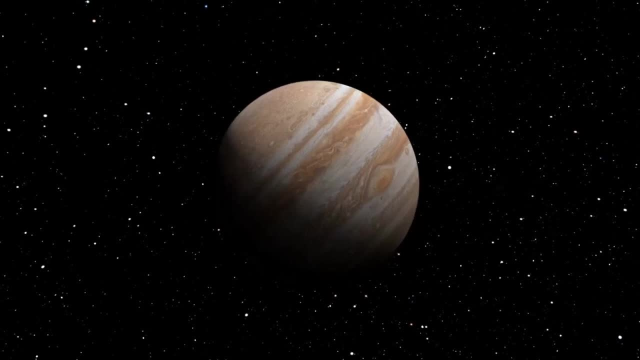 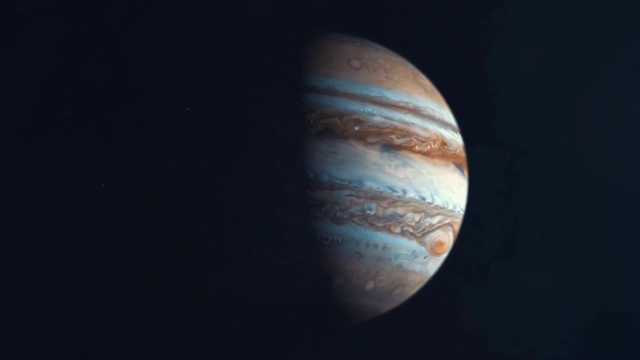 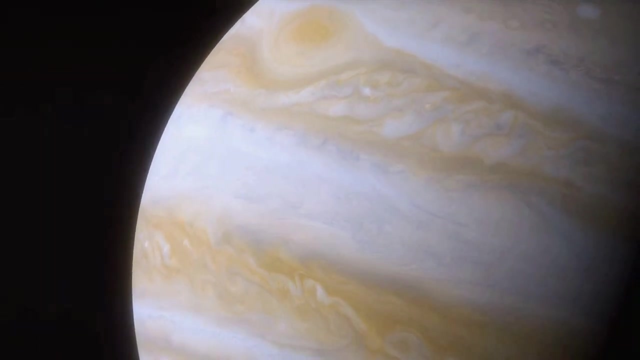 This potential habitat makes Europa one of the most promising places to look for life beyond Earth. Ganymede, the largest moon in the solar system, is even bigger than the planet Mercury. It's the only moon known to have its magnetic field. Ganymede's surface is a mix of two types of terrain – dark, heavily cratered regions. 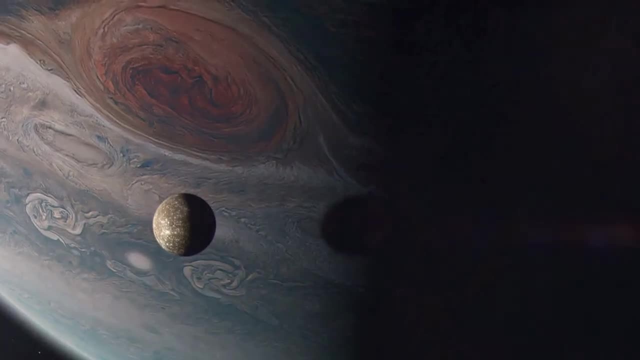 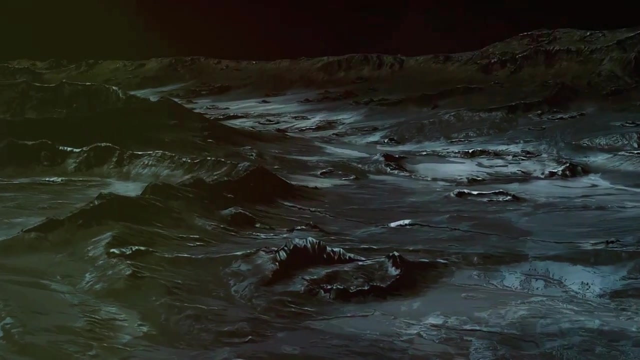 and lighter, younger regions, marked with an extensive array of grooves and ridges. And last but certainly not least, is Callisto. This heavily cratered moon has the oldest, most heavily cratered surface in the solar system, a testament to the cosmic battles it has survived over the eons. 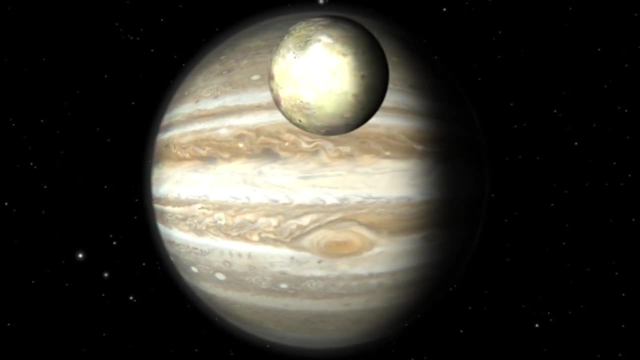 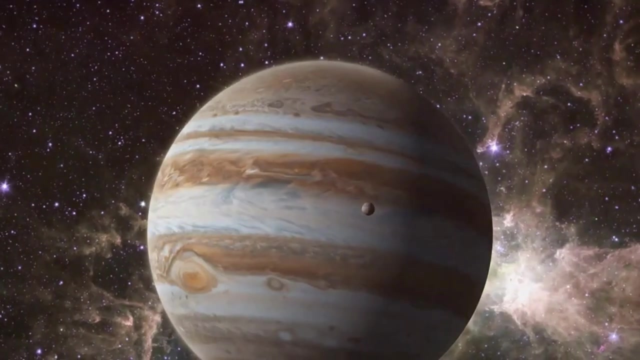 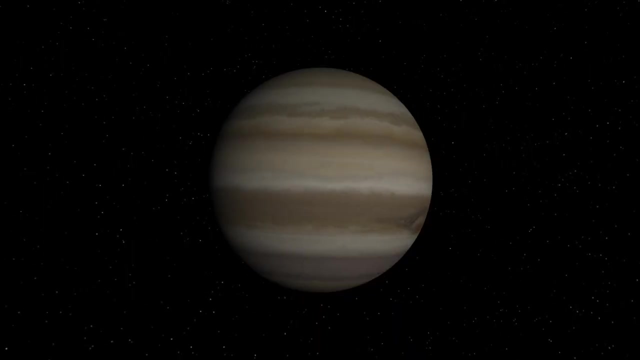 Each of these moons, with their unique geology and potential for life, contribute to the rich and diverse family that orbits Jupiter. They are a testament to the planet's gravitational might and its standing as the reigning monarch of our celestial neighborhood. With such a diverse array of moons, Jupiter holds the crown for the planet with the most. moons. As we conclude our cosmic journey, we take a moment to reflect on the vast majority of the fascinating discoveries we've made. We've journeyed to Mars, the red planet home to two moons, Phobos and Deimos. that.